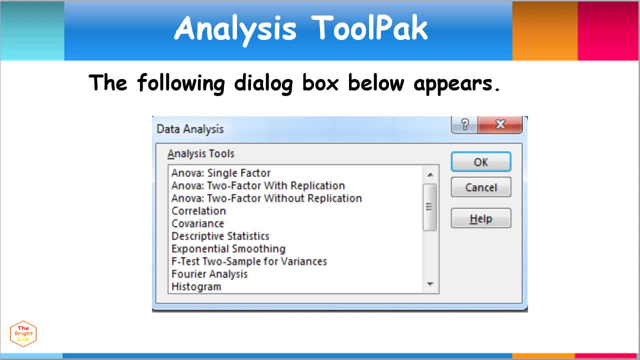 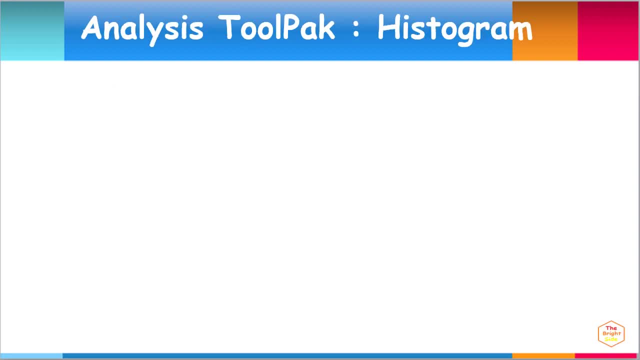 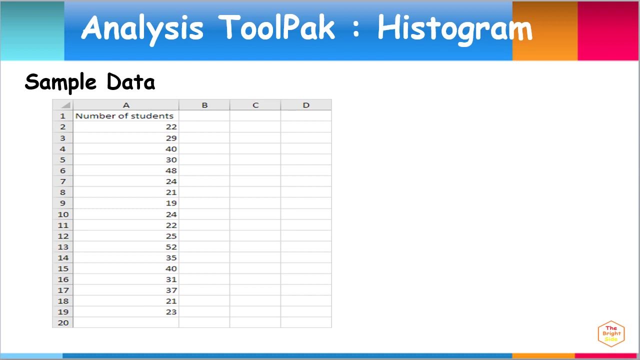 From all the different choices available here, we can now select which data analysis tools we need. Let's have a practical example. For instance, we want to have the histogram for our data. The histogram is a very useful data analysis which is available in the Excel analysis tool. 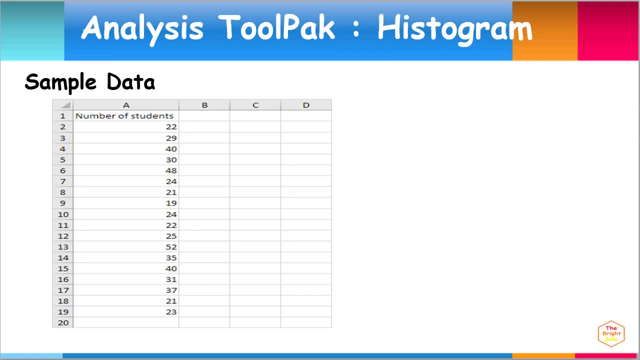 pack. Let's use this sample data During data analysis. data can be grouped based on specific intervals. In this case, data can be grouped to 0 to 20,, 21 to 25,, 20 to 25,, 20 to 25,, 20 to 25,. 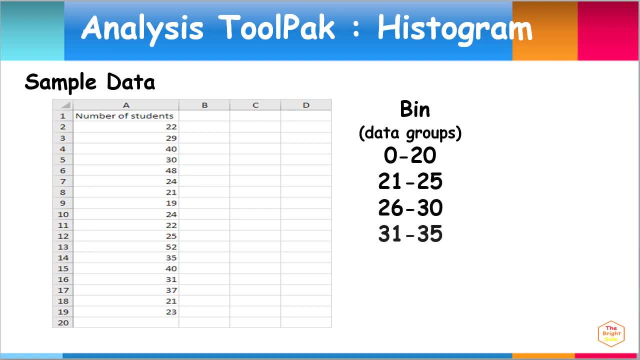 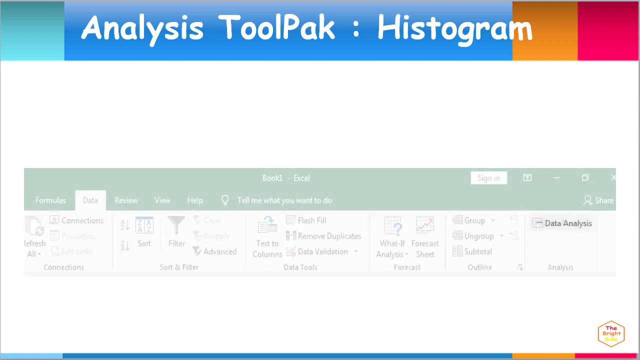 26 to 30,, 31 to 35, and 36 to 40. The corresponding bin numbers represent the upper levels for each data groups. So let's now use the Excel analysis tool pack to get the histogram for our data. 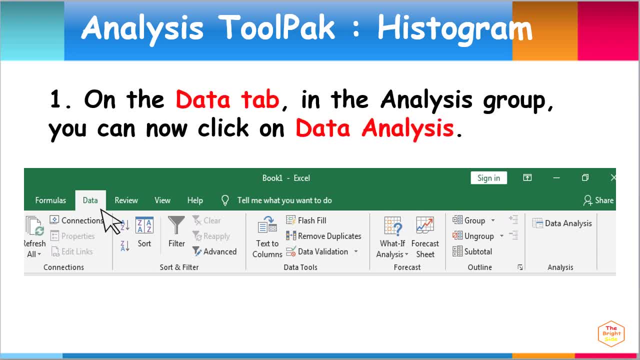 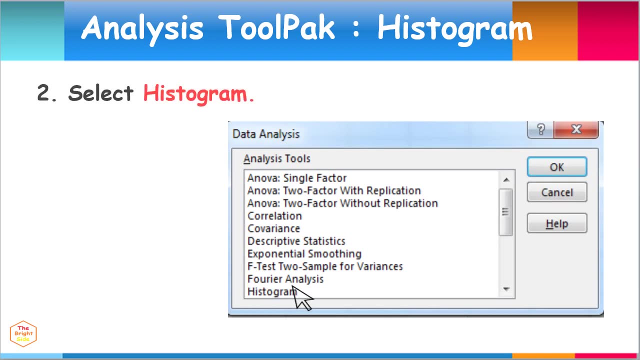 First click on the data tab. Then in the analysis group you can now click on the data analysis and you can now see what ederim. On the data analysis dialog box, select histogram, Select this value data. Then on the data 테- ㅋㅋㅋㅋ. in buyers database, underoster G, we can select our data. 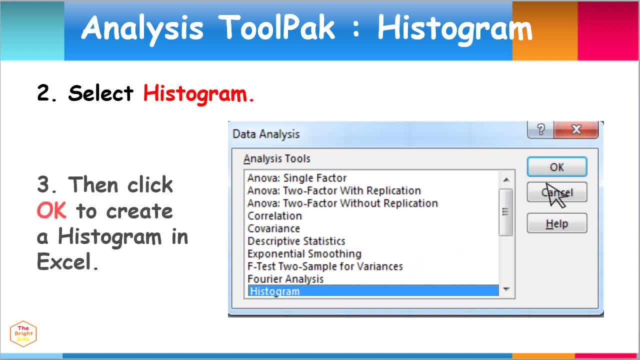 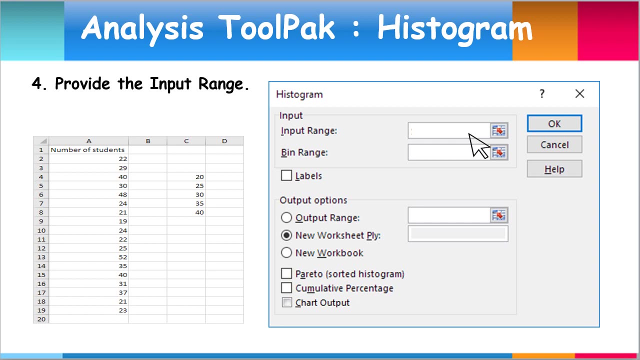 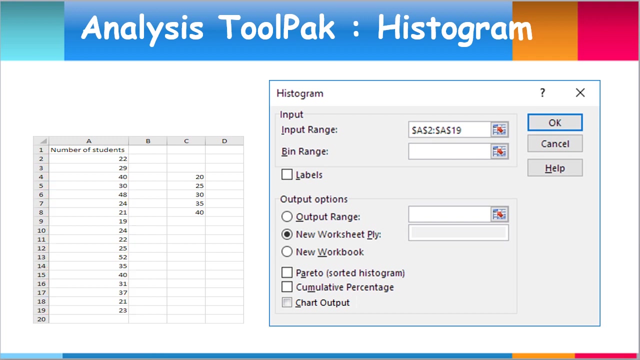 Then click OK. This will create a histogram in Excel. Next is to provide the input range. To do this, simply select the cell range from A2 to A19, found in the table of our sample data. Then provide the bin range. 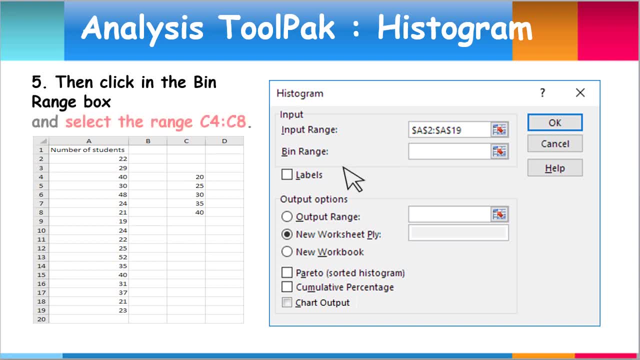 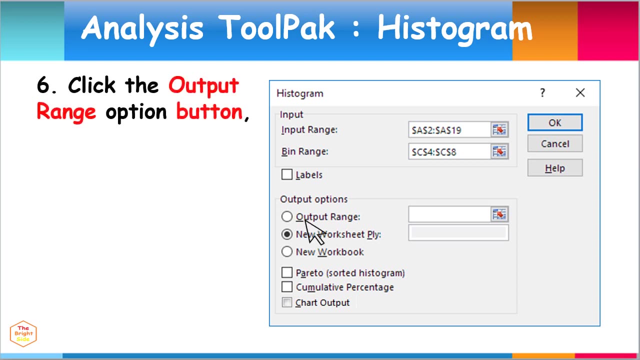 To do this, click in the bin range box and select the cell range from C4 to C8.. These are the bin numbers that represent the groupings of data. Next click the output range option button, Then click in the output range box and then select cell F3.. 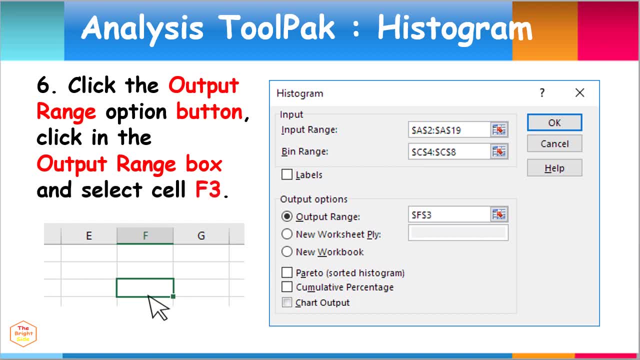 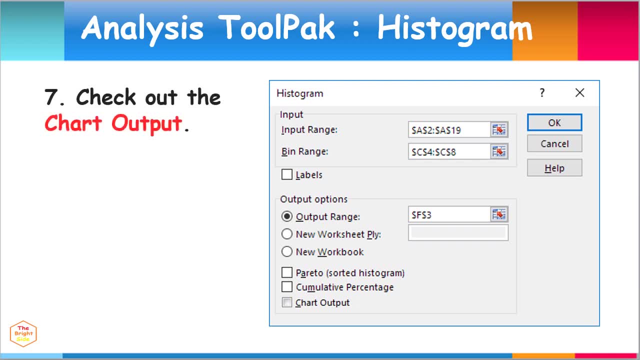 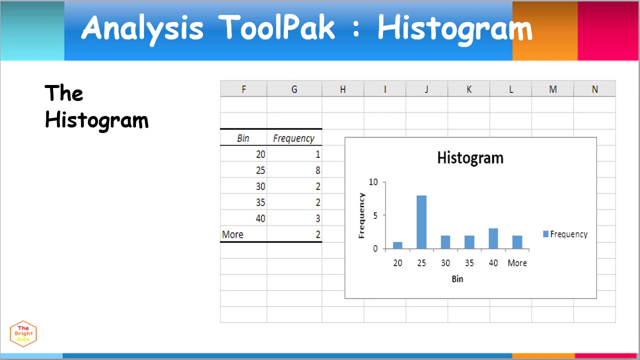 This provides the location placement of the resulting histogram. Also, make sure to check out the chart output radio button found on the bottom part of the dialog box, Then click OK. Here's the histogram for our sample data. It's a graphical display of data using bars of different heights. 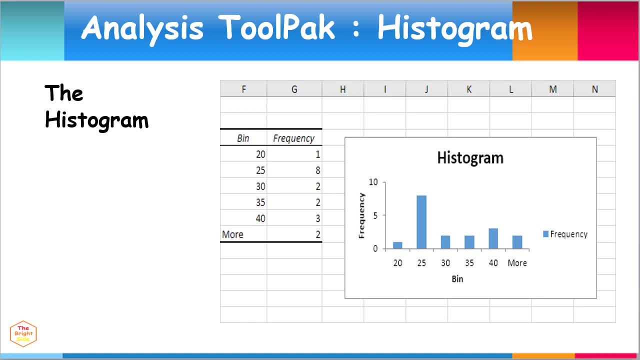 It is similar to a bar chart, but a histogram groups numbers into ranges represented by bin numbers. The height of each bar shows how many fall into each range. Next click in the input range box. You can see that the bar chart is shown as the frequency. 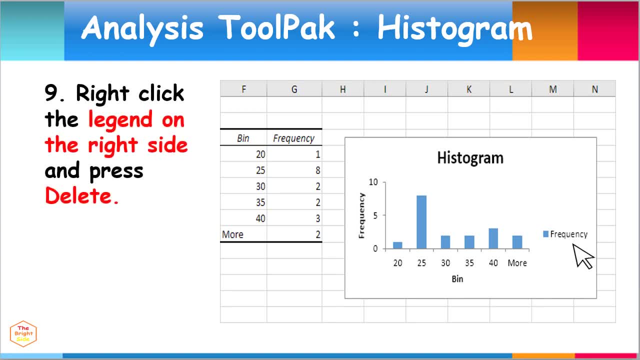 Then you may right-click the legend on the right side and press delete. Also, it is best to properly label the chart by changing bins to number of students. There is also the option to remove the space between the bars. To do this, just click in the input range box and then click in the input range box. 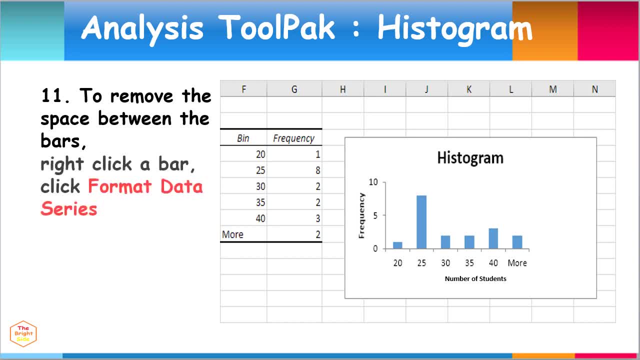 and then click in the input range box. To do this. click in the input range box and then click in the input range box and then click in the input range box To add borders: just right-click a bar, click Format Data Series and change the gap width. 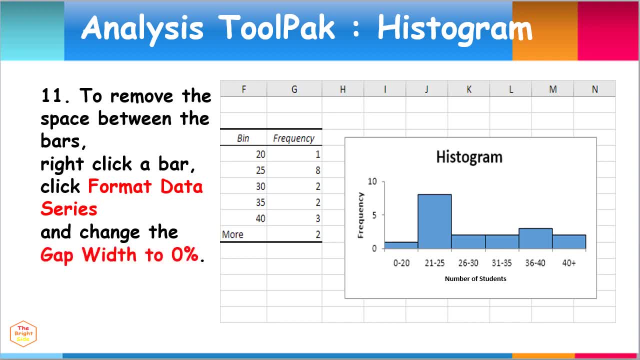 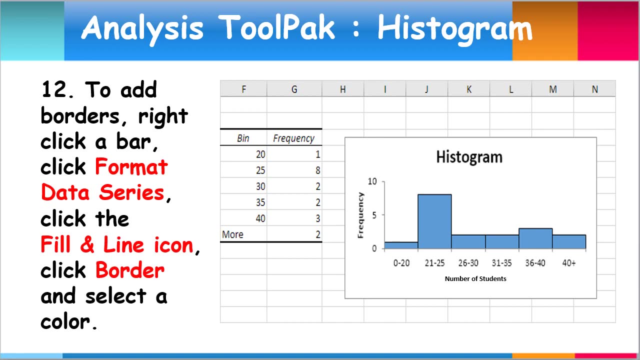 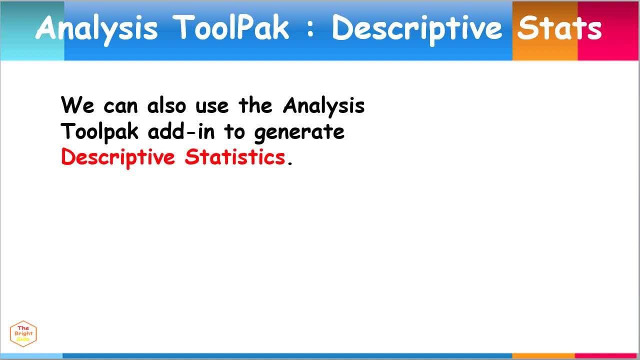 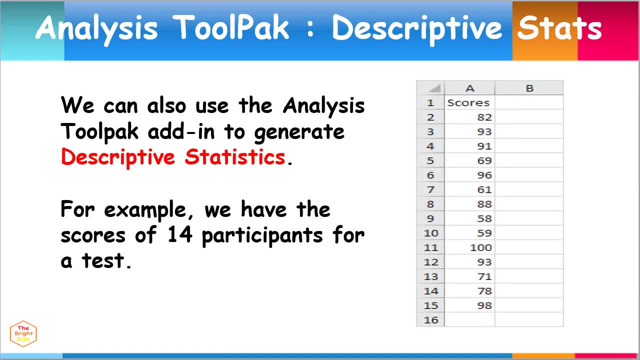 To add borders: just right-click a bar, click the Fill and Line icon and select a color To generate descriptive statistics from the given data. For example, we may have the scores of 14 participants for a test as our sample data.